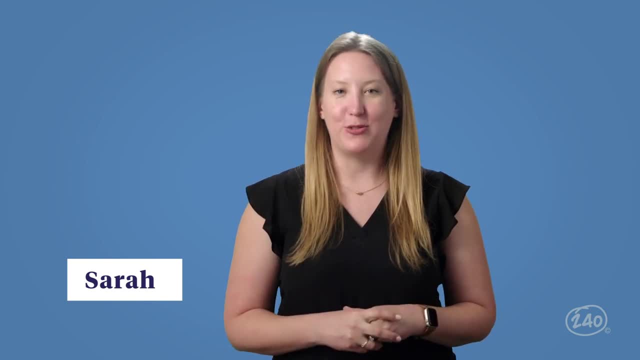 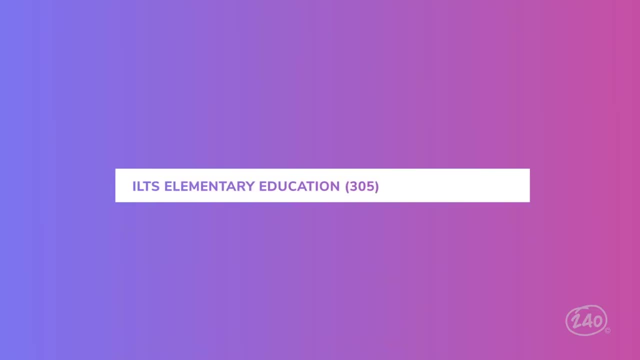 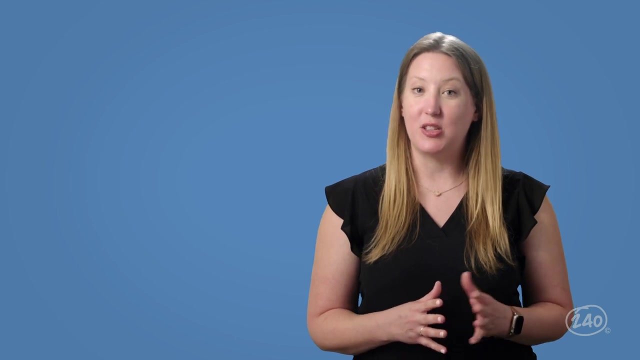 teaching Illinois students in the classroom, and now I work with 240 to help teachers pass their certification exams. And today I'm going to help you. This video is going to prepare you for the Illinois Elementary Education Exam. That's test code 305.. This is a test for teaching grades. 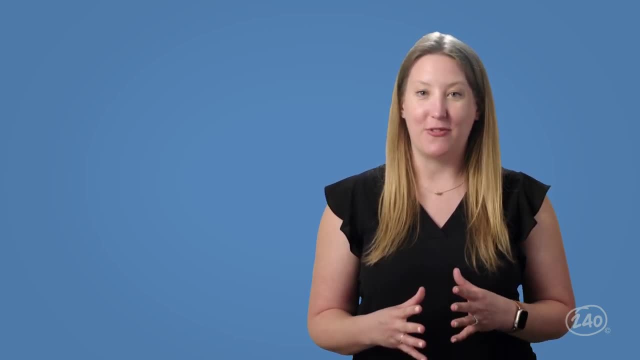 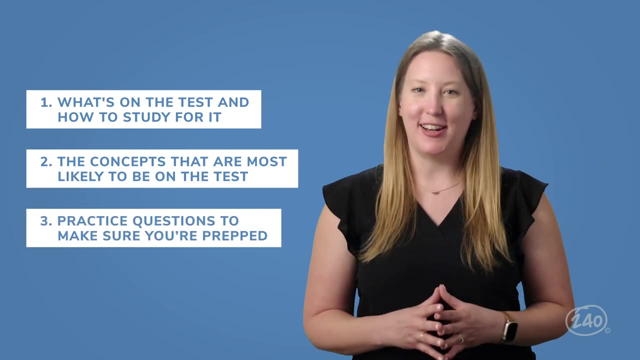 one through six in Illinois, And this video is going to cover three things: What's on the test and how to study for it, The most important concepts to master, And we're going to look at a few practice questions. The Illinois Elementary Education Exam covers six sub areas. 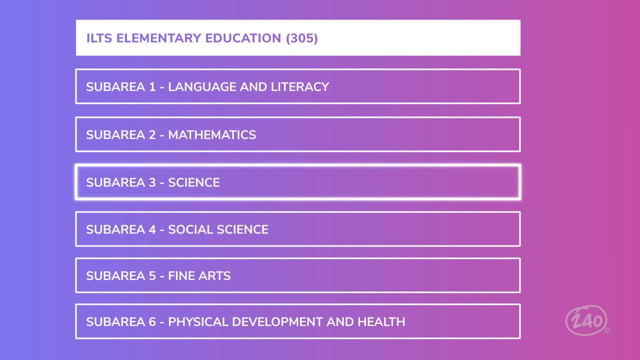 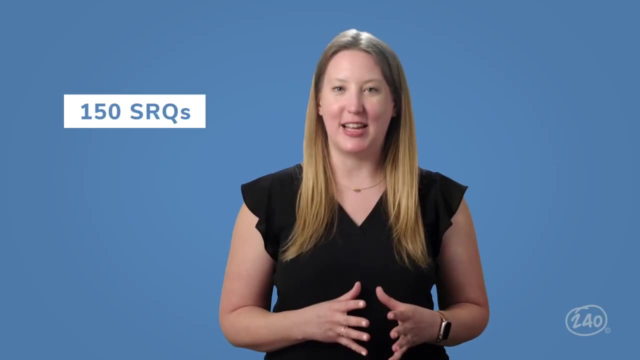 language and literacy, mathematics, science, social science, fine arts and physical development and health. Each is worth a certain percentage of your exam, So each contains a specified number of select response questions. You'll have 150 select response questions to answer in all. Each sub area is broken down further by objectives. 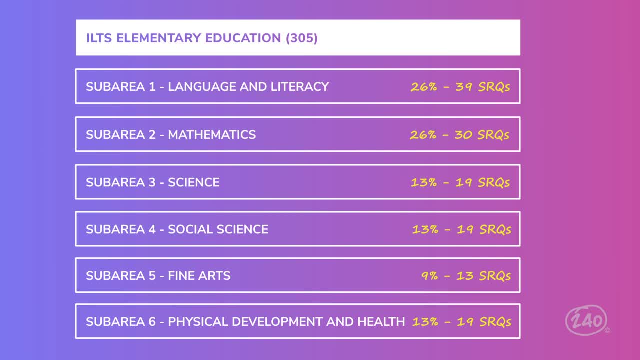 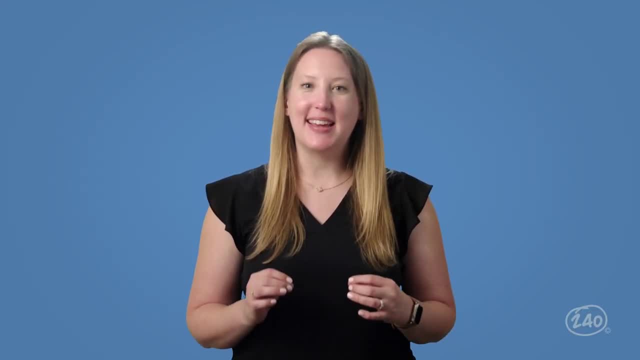 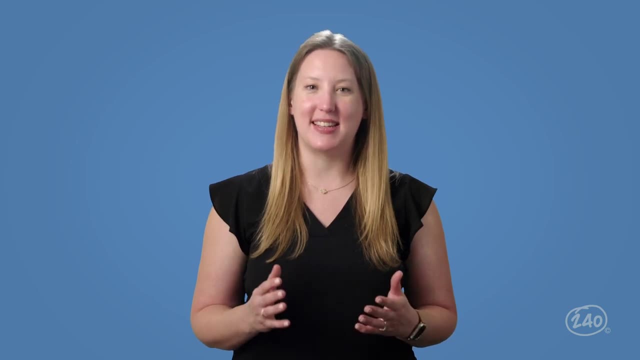 We'll overview each sub area, then dive into a key concept that you'll need to know for your exam. Let's take it from the top with language and literacy. This is one of the biggest sub areas on the exam, accounting for 26% of the overall score, And it's comprised of six objectives. 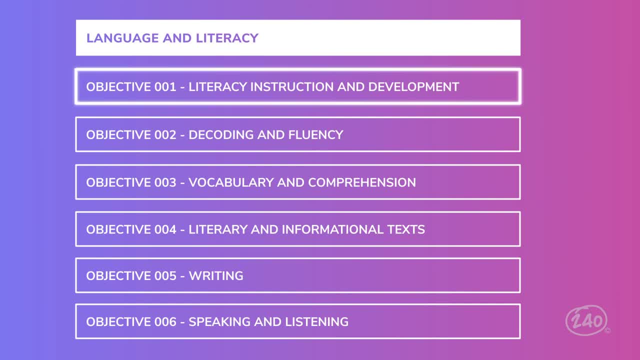 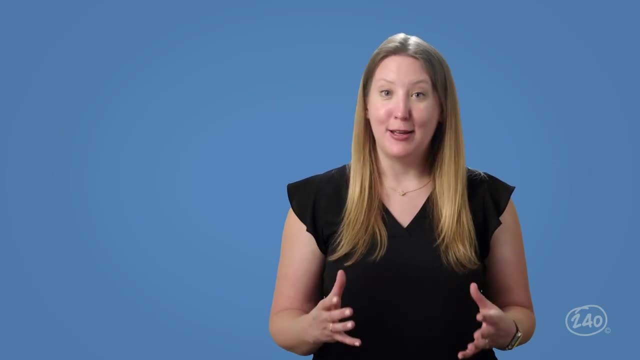 Let's take a look at those. now You'll tackle literacy, instruction and development, decoding and fluency, vocabulary and comprehension, literary and informational texts, writing and speaking and listening. Now, that may sound like a lot, because it is, But we have everything. 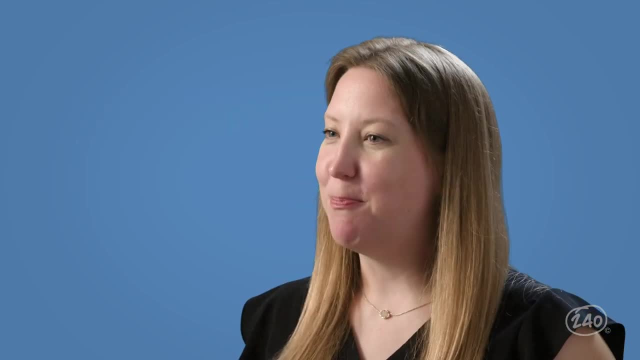 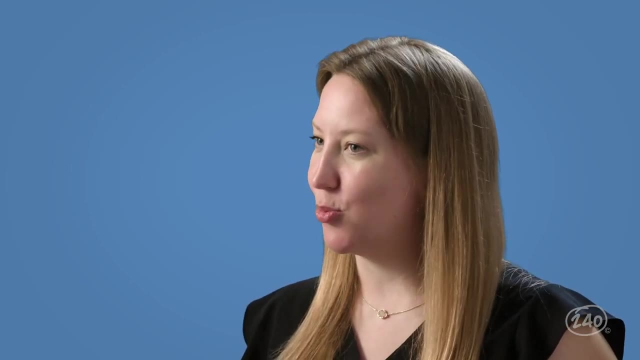 in our study guide. The link to subscribe is below. But if you want to stick with me for now- and I don't blame you, I am pretty fun- I'm going to go over an important concept right now. You'll need to be able to teach students to determine the meaning of unknown words. they 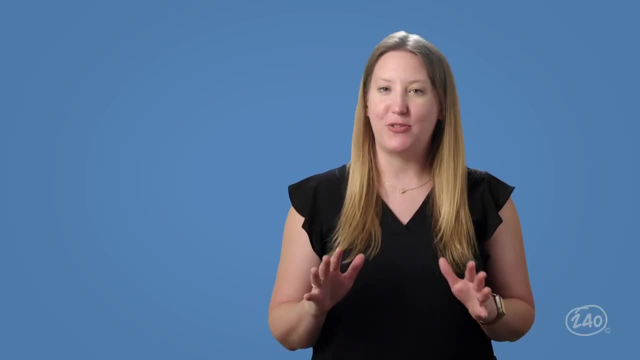 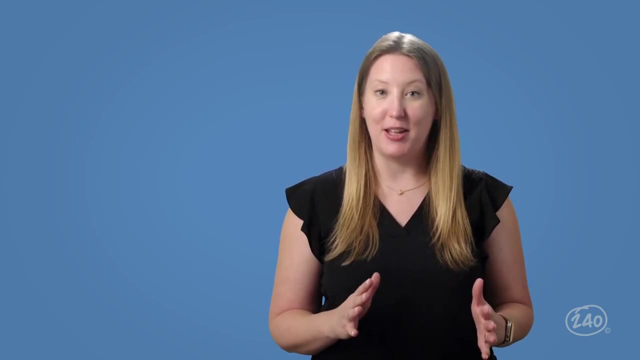 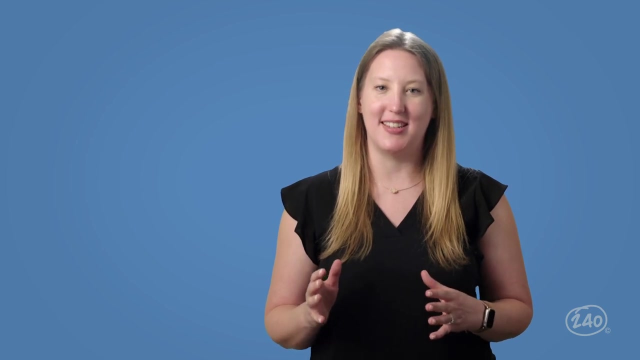 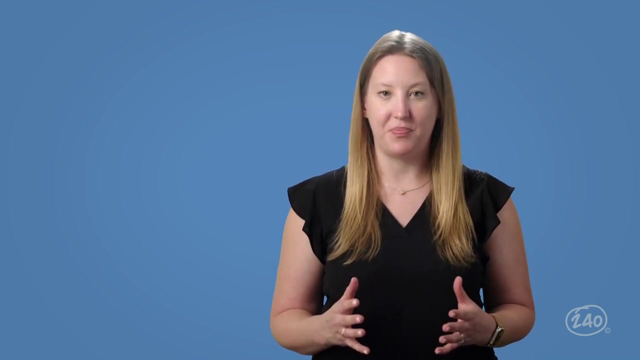 come across while reading. There's a time and a place for direct vocabulary instruction. in the classroom, However, indirect vocabulary instruction is common, So strong readers also need strategies for determining the meaning of unknown words they come across in text. Morphemic analysis and contextual analysis are two such strategies. We'll go over morphemic analysis. 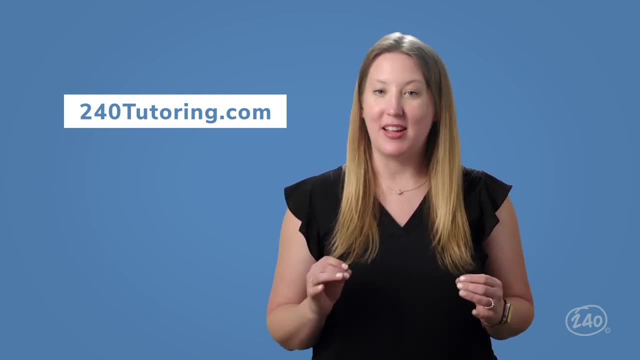 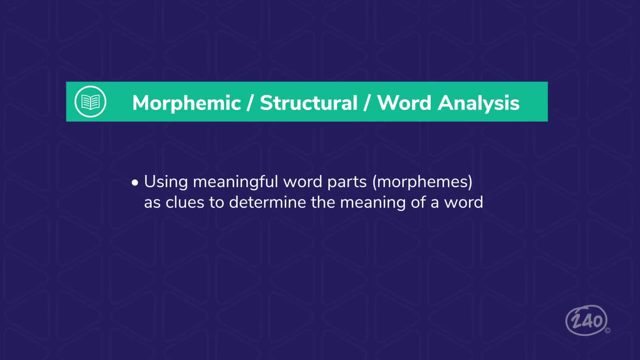 right now, But if you want to see all the information about contextual analysis too, check out the study guide. Morphemic analysis, also known as structural analysis or simply word analysis, is used to determine the meaning of unknown words that come across in text. 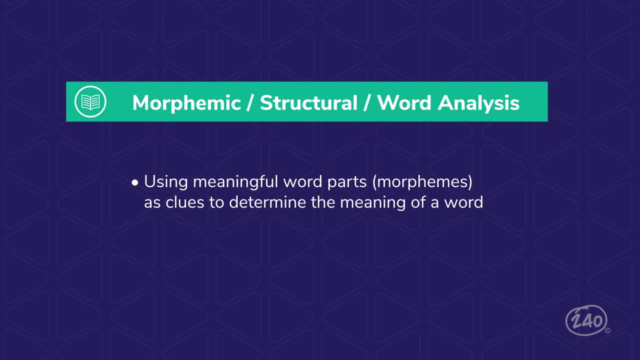 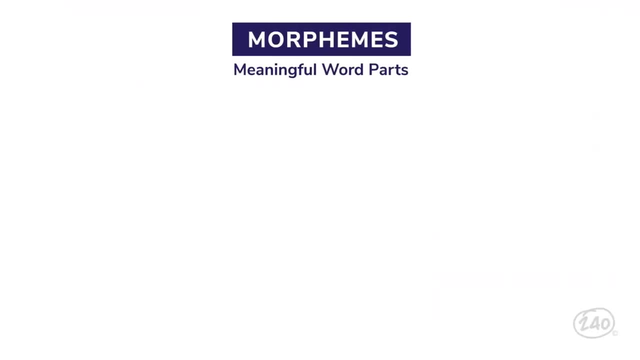 Using meaningful word parts known as morphemes, as clues to determine the meaning of a word. Let's take a deeper dive into morphemes. We can categorize morphemes as roots and affixes. Roots are the basis to which affixes may be attached. They provide the core meaning of a word. 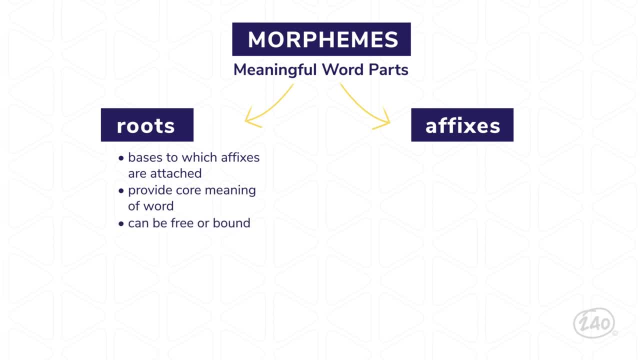 A root may be free, meaning it can stand alone as its own word, or bound, meaning it cannot stand alone. Examples of roots that can stand alone include those derived from the Anglo-Saxon language, such as help, love and friend. Examples of roots that cannot stand alone include Greek and Latin. 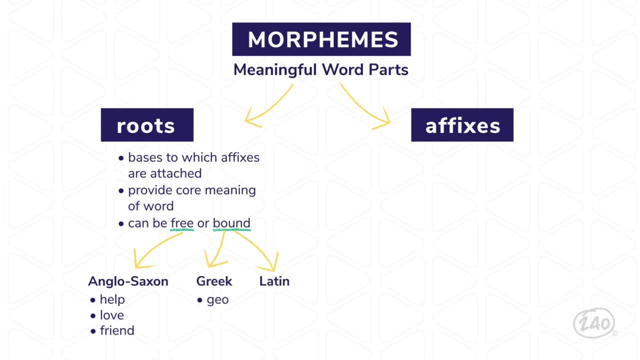 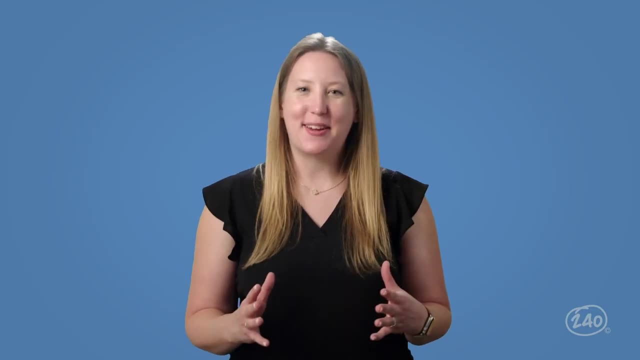 Geo, meaning earth, is an example of a Greek root. It can be found in words such as geography and geology. Omni, meaning all, is an example of a Latin root. It is part of words like omniscient and omnivore. Now let's take a closer look at affixes. 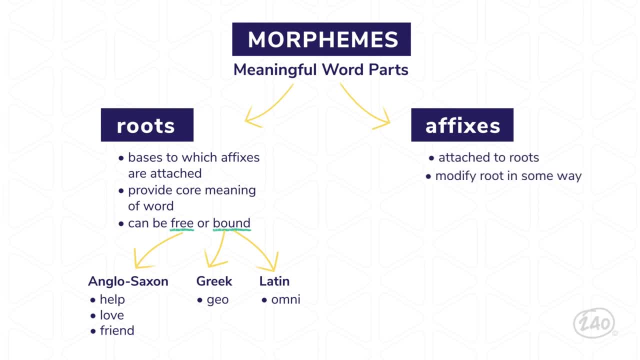 Affixes are morphemes that can be attached to roots to modify them in some way. An affix cannot stand alone as its own word. Affixes can be categorized as prefixes and suffixes. A prefix comes before the root of the word. Examples include un- re- and dis-. The suffix comes after the root of the word. 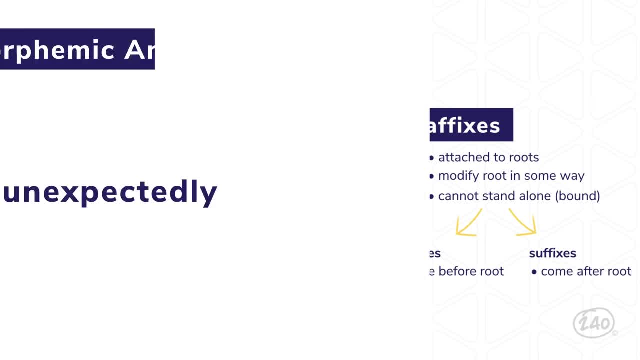 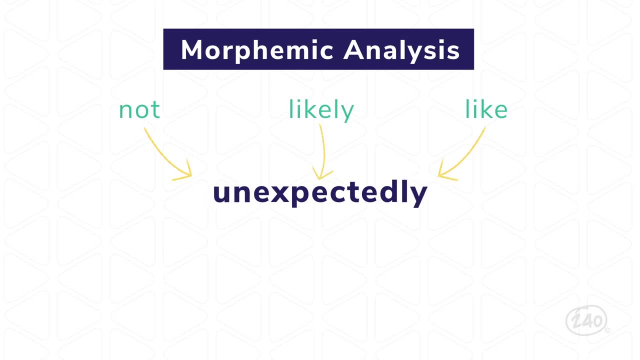 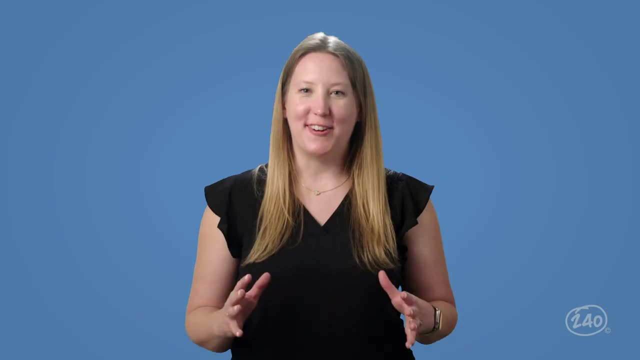 Some examples are ed- ful- and ing-. When readers break words into meaningful parts, determine what those parts mean and put them back together to determine the meaning of the whole word, they're using morphemic or structural analysis. All right, let's move into the math sub. 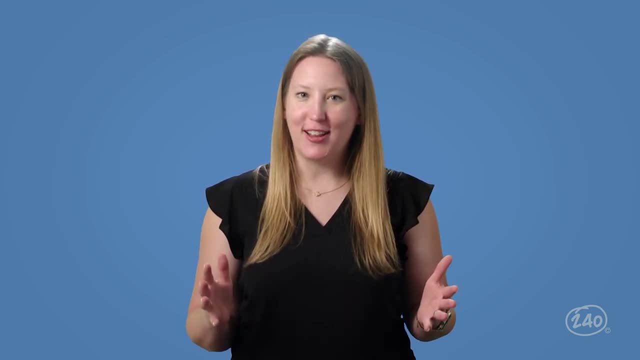 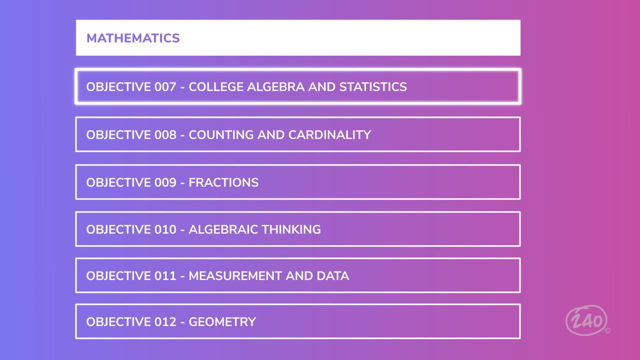 area, which is also worth a big chunk of the overall exam at 26% For the mathematics sub area. you'll need to know all about algebra, math and math. You'll need to know all about algebra, math, algebra and statistics, counting and cardinality fractions, algebraic thinking. 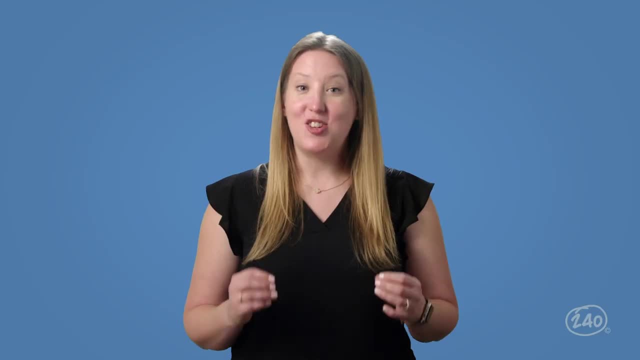 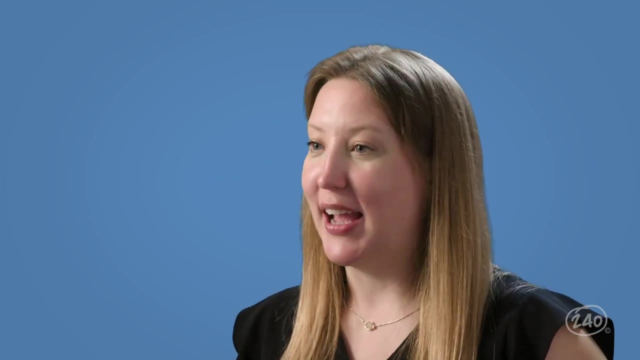 measurement and data and geometry, And just like in the language and literacy sub area. if that sounds like a lot, it's because it is, But don't worry, I'm going to pick out a couple of important things to touch on right now, For example in the college and algebra statistics. 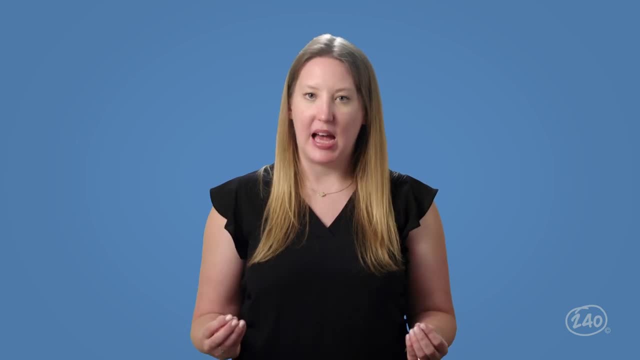 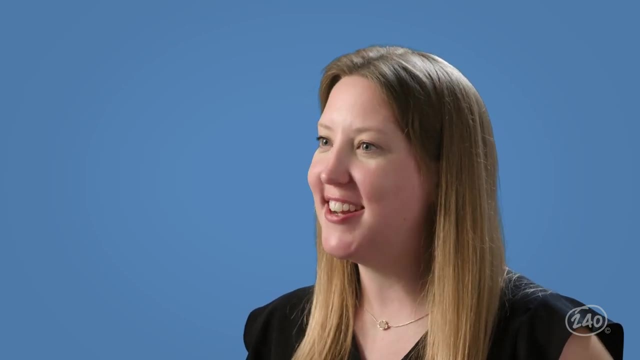 objective. the measures of center and range come up a lot. Need a quick refresher here. Sounds like a great opportunity to peek into our study guide, where we've got tons of videos meant to teach or reteach everything you need to know to pass, Roll the tape. 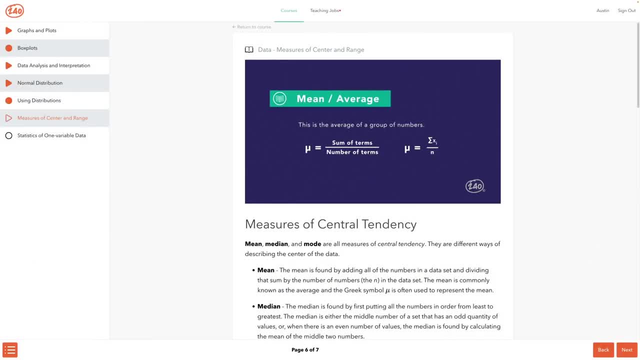 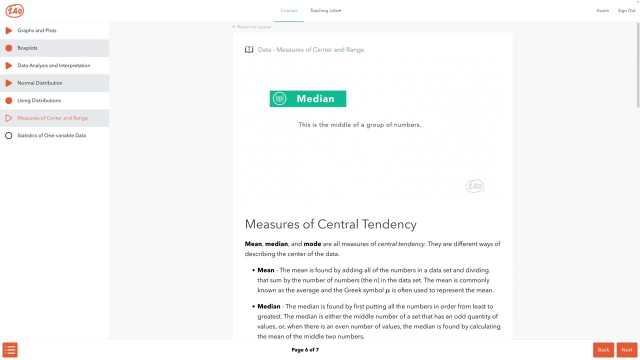 The mean is more commonly known as the average. It is often represented by the Greek letter mu and is calculated by dividing the sum of the terms by the number of terms. To find the median, start by ordering the numbers from least to greatest. In a set that has an odd number of terms, the median is the middle value of that. 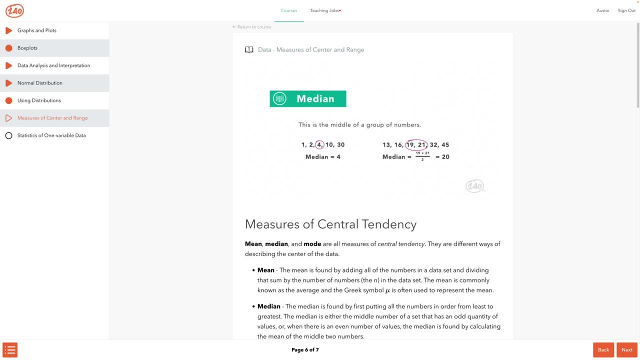 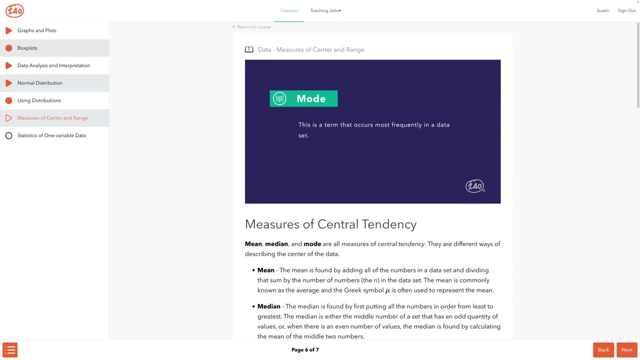 set When there is an even number of terms. the median is found by calculating the mean of the middle two numbers. The mode is the term that occurs most frequently in a data set. Some sets of data have no mode. This occurs when all terms share the same frequency. 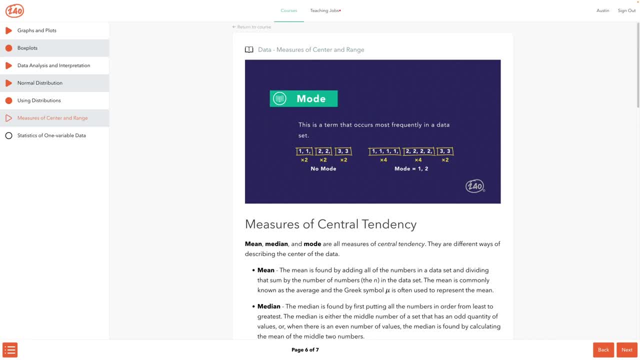 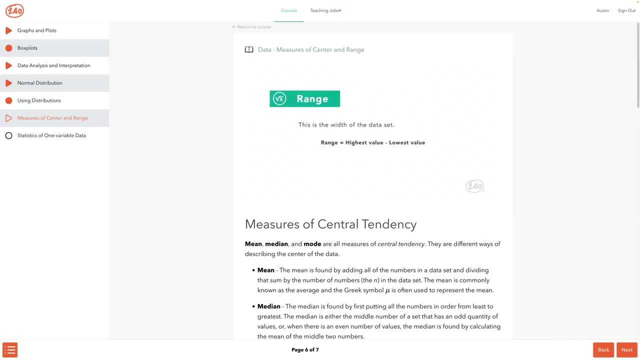 Some sets of data have more than one mode. This happens when multiple pieces of data in a set appear the same number of times and appear more than any other data values. The range is the difference between the highest data value and the lowest data value. In general, the greater the range, the more spread out the data is. 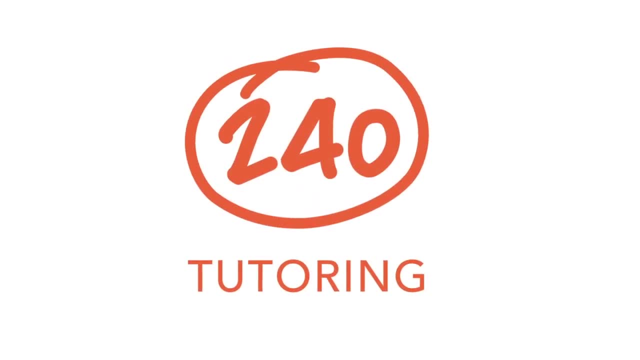 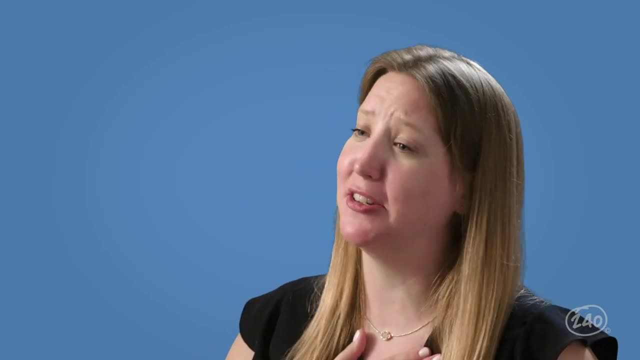 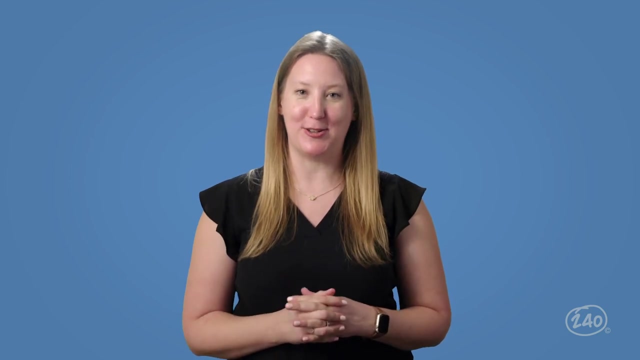 The smaller the range, the more it clusters together. Wow, I just love a good educational video And at the end, when she explained range, get it together. Sarah, We've got a lot of math to talk about. How about we look at a little geometry? You're going to want to brush up on common line and 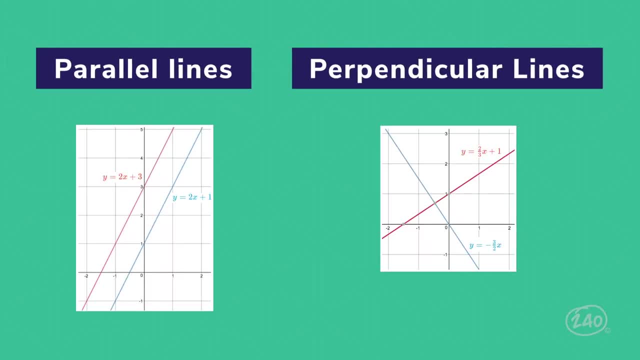 angle relationships. When we say line relationships, we mean whether lines are parallel, meaning they never intersect, or perpendicular, meaning they intersect at a 90 degree angle. And you can tell if lines are parallel or perpendicular by looking at their equation in slope-intercept form, which is: y equals mx plus b. 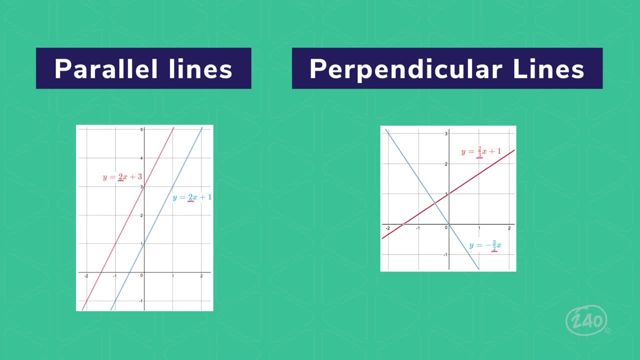 M is the value for slope. We've got it written out here for you already. Parallel lines have the same slope, Since both of these lines have a slope of two. they're parallel. Perpendicular lines have slopes that are the opposite reciprocals of each other, Since one line has a slope of two-thirds and one has a slope of. 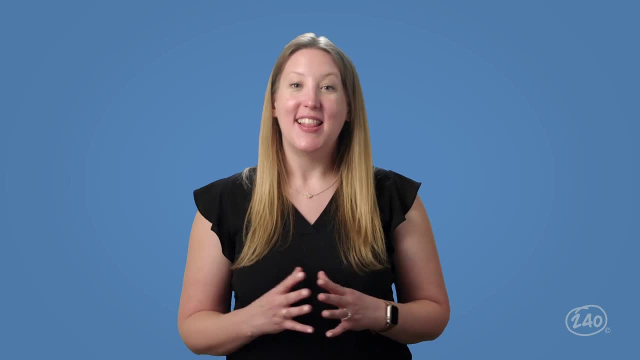 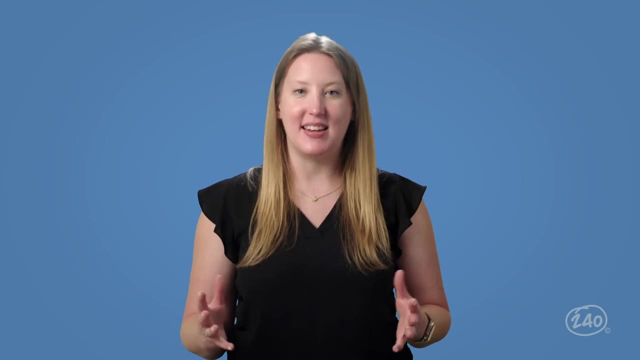 negative three-halves. they're perpendicular. Lines can also be neither parallel nor perpendicular, which just means they intersect at an angle that is not 90 degrees. No matter what objective we're looking at, it's important that you not only know the content. 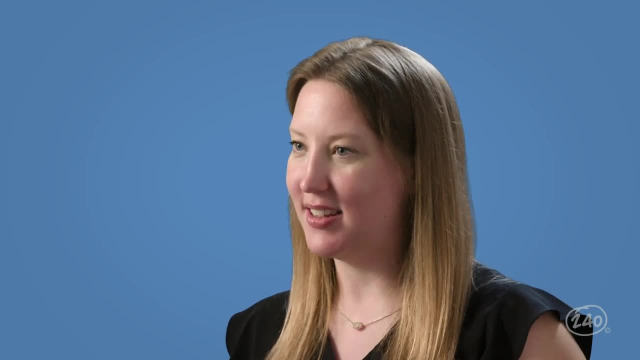 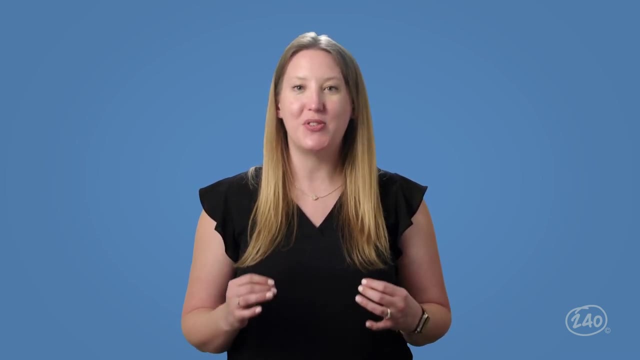 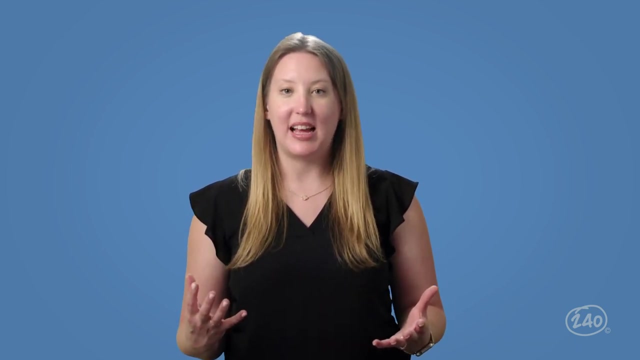 but also how to interpret it. So let's take a look at this: How to teach the content to your students. Understanding how kids learn math includes mastering a variety of teaching strategies that improve student understanding, like how to incorporate manipulatives and other tools like calculators into your lessons. 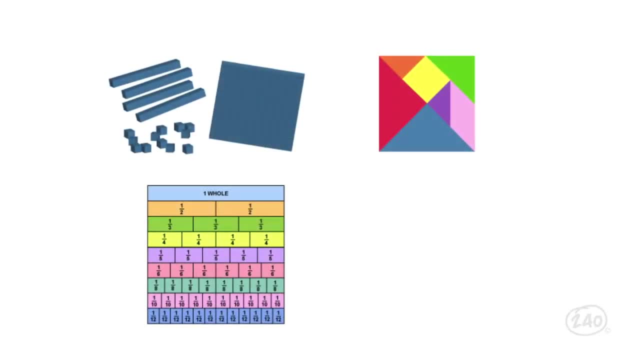 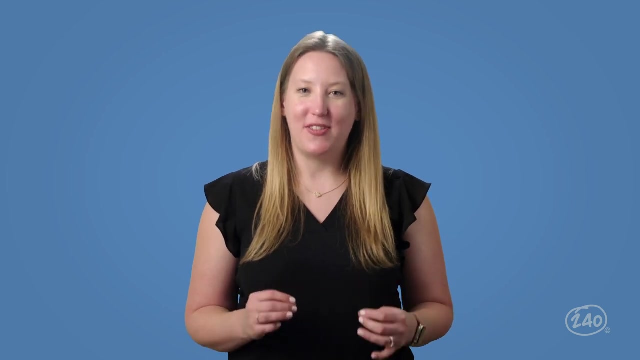 Counting blocks, tangrams, fraction tiles and color counters can all be used to enrich students' understanding of mathematical concepts. You need to understand what they are and when it is appropriate to use them. So, for example, if you're working on Objective 9. 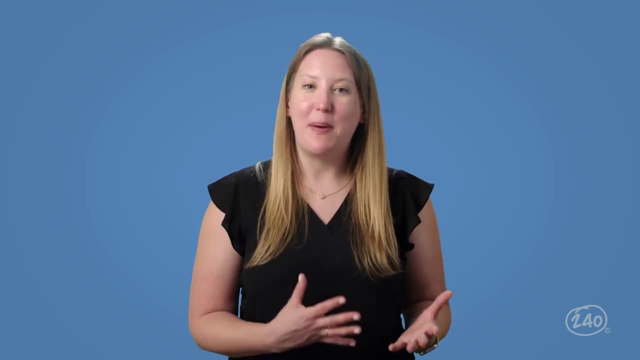 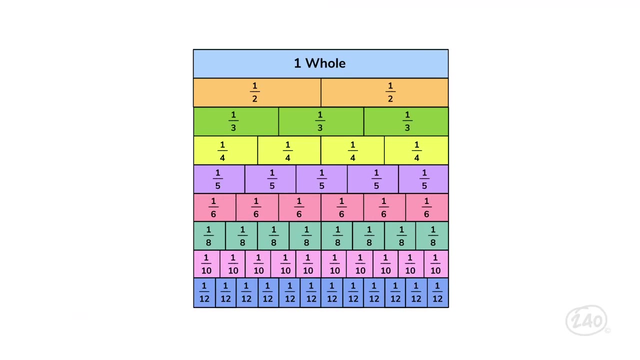 and dealing with fractions. you may be asked what manipulative best helps students understand that two-fourths is equal to one-half. Fraction tiles would be the best choice because students could see that together, two one-fourth tiles are the same size as one-half tile. 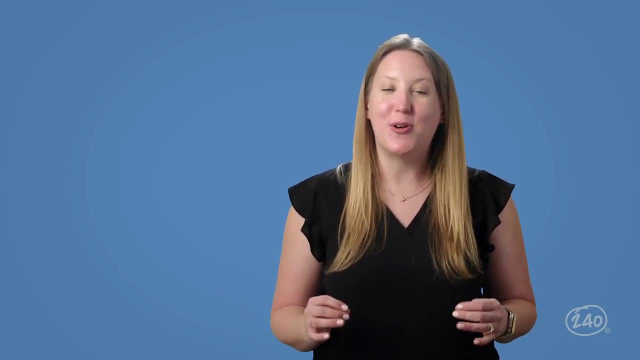 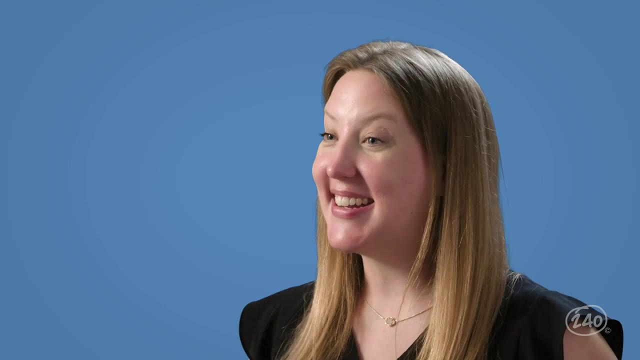 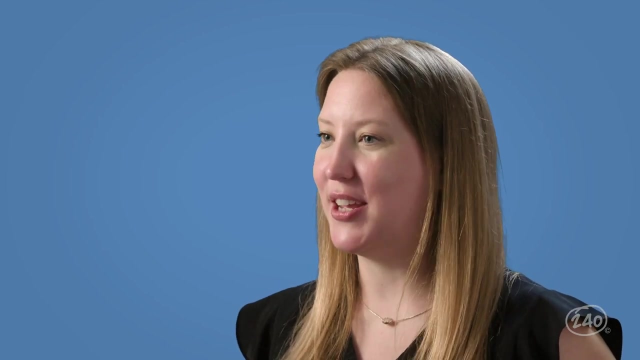 That about wraps up math, But remember there is so much more that we didn't have here, so if you're still feeling a little nervous, go check out our study guide On to science. Science only makes up about 13% of this exam, but that's still a solid 15 questions. 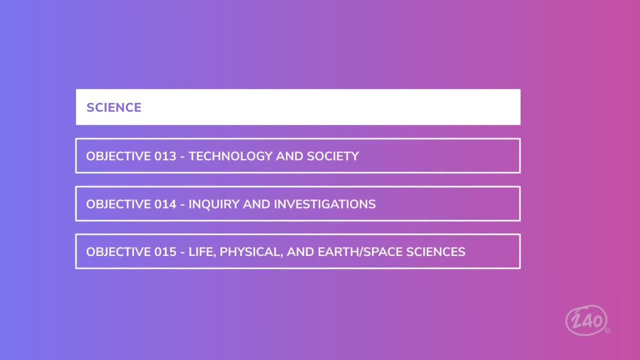 so you'll want to make sure you brush up In the science section. you'll need to understand the relationships between science, technology and society. You'll use your investigation and inquiry skills and understand life, physical and earth and space science. That first objective can be kind of tough to understand, so let's break it down. 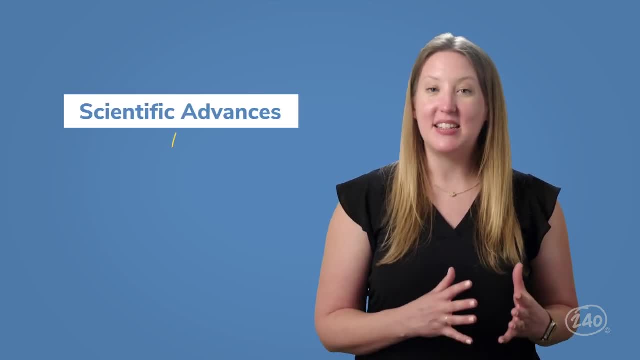 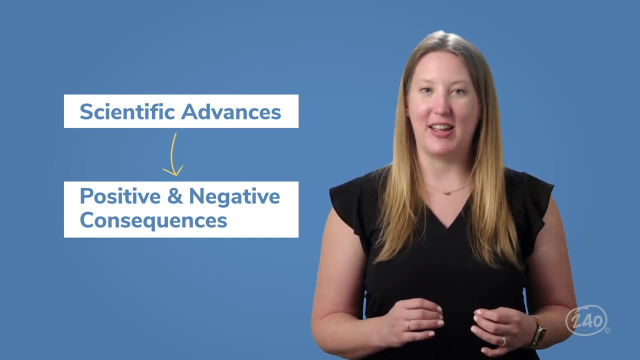 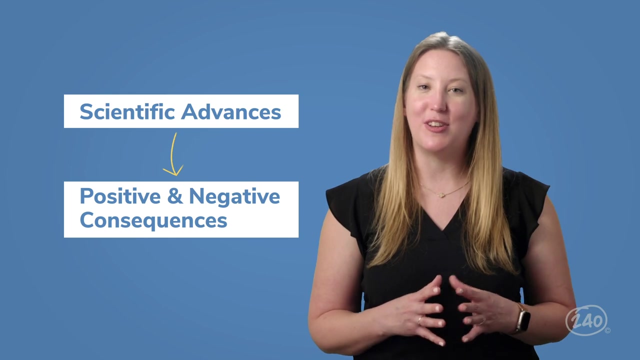 You'll need to know both how scientific advances lead to major improvements, like the combustion engine, the internet and stem cell technology, but also how advances in technology have led to increased greenhouse gas emissions and the ethical considerations surrounding different types of experimentation. Another hot topic here: renewable. 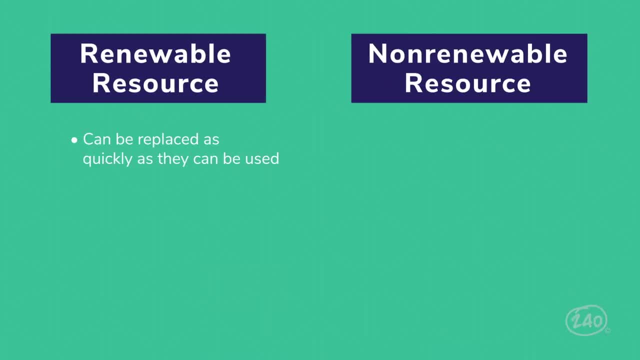 resources. Renewable resources can be replaced just about as quickly as they can be used. They include green energy, such as water and wind, and solar energy, which comes from the sun, and commodities such as drinking water, crops and wood, While non-renewable resources are gone. 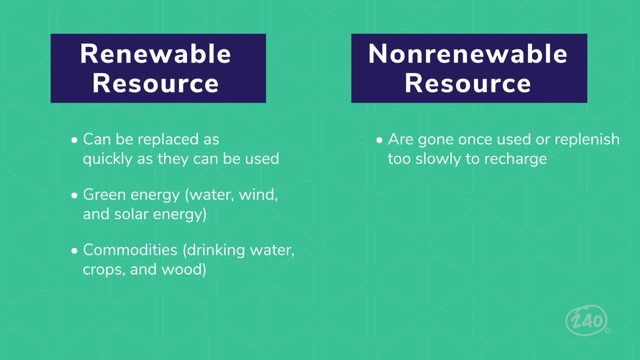 once used or replenished too slowly to recharge. they include fossil fuels such as coal, oil and natural gas, and minerals such as nitrogen, carbon dioxide and carbon dioxide. They also include a lot of resources such as gold, iron ore and titanium. You'll also need to know the basics. 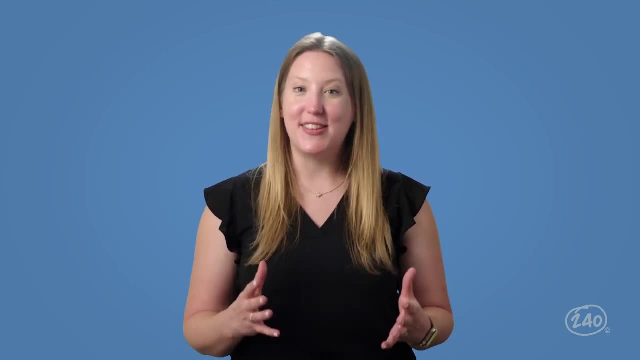 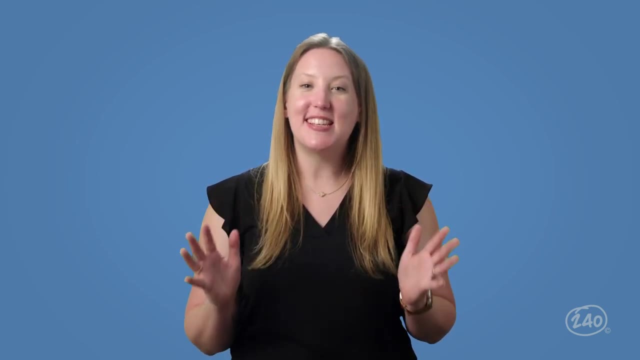 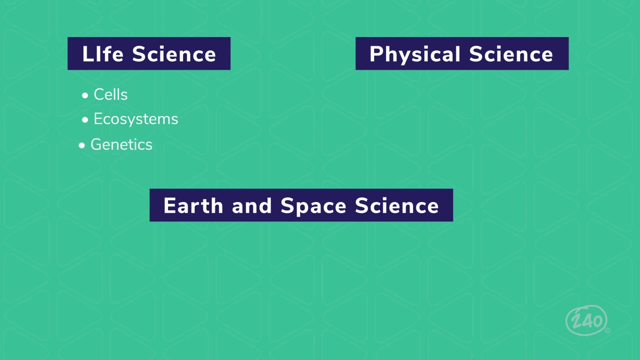 from each branch of science- life science, physical science and earth and space science- And since I don't have time to walk you through each one, let me just list a few highlights for you. In the life science section, you'll want to know about cells, ecosystems and genetics. 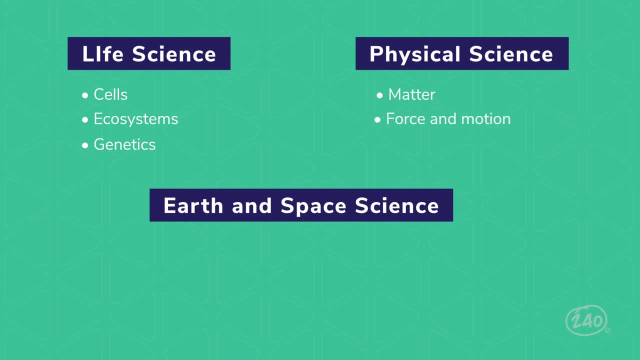 For physical science, focus on matter, force in motion and energy. And in the earth and space science section, you'll need to know the structure and composition of earth, earth's location in the universe, and weather and climate. And then don't forget, 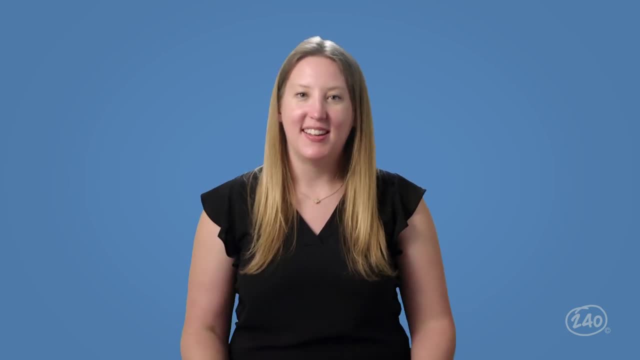 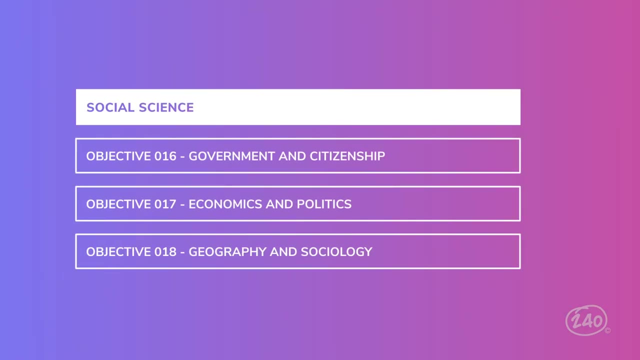 you'll need to know how they all fit together. That about wraps up science. How about we take a look at social science? The social sciences sub-area makes up about 13% of the total exam and that's another 15 questions And it contains three objectives. The first is to know the 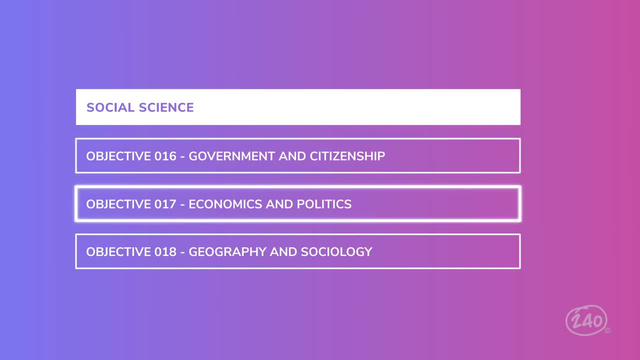 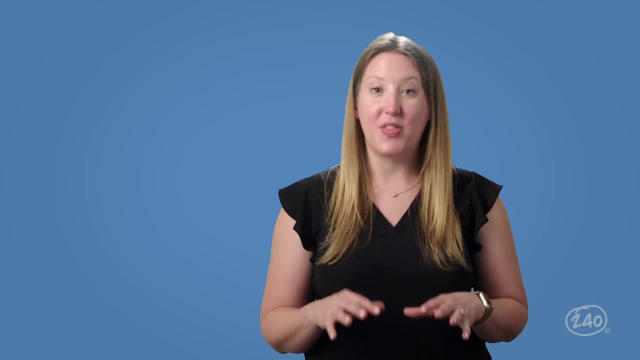 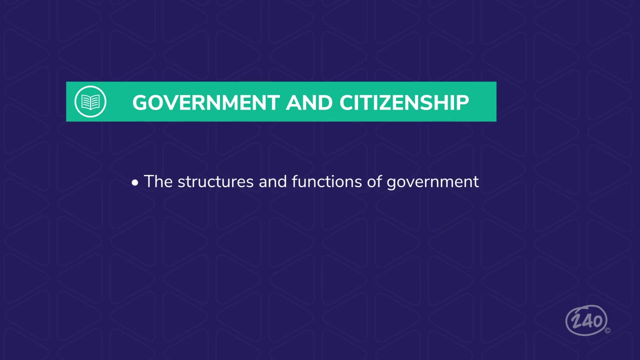 objectives: Government and citizenship, economics and politics, and geography and sociology. Let's briefly cover what you might expect to see on the exam for this sub-area, starting with government and citizenship. The objective breaks down into three primary areas. you'll need to understand The structures and functions of government at the federal 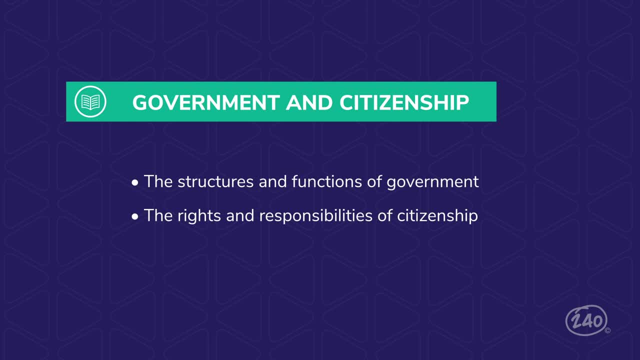 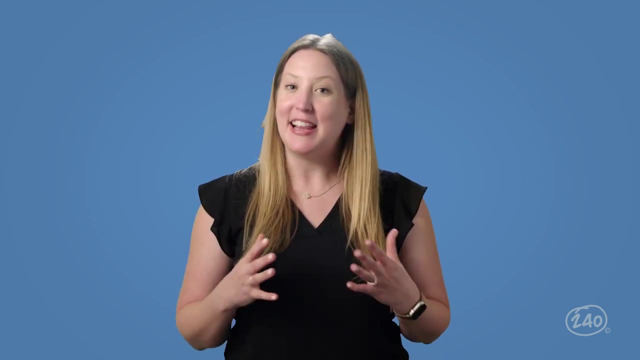 state and local levels, The rights and responsibilities of US citizens And the skills, knowledge and attitudes that a successful American should possess. For example, you may be asked to identify a key principle in an important American document like the Bill of Rights or the Gettysburg Address, Or you may be asked to apply principles of citizenship. 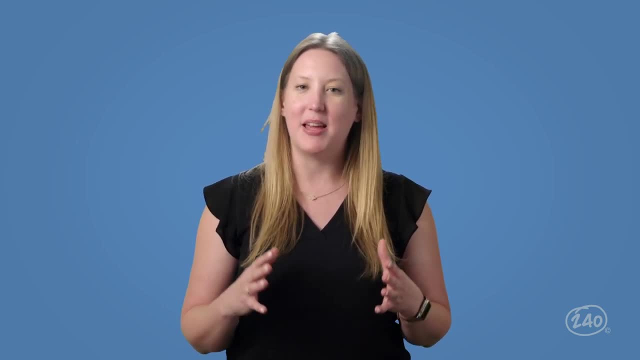 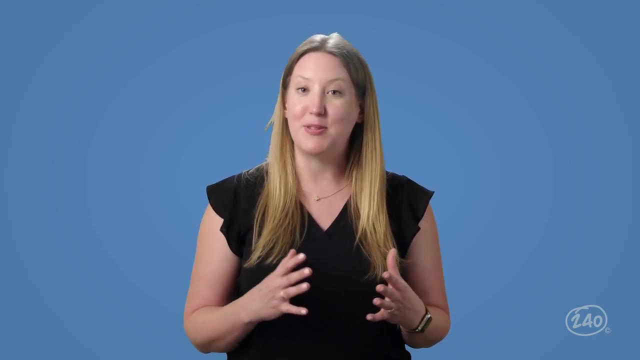 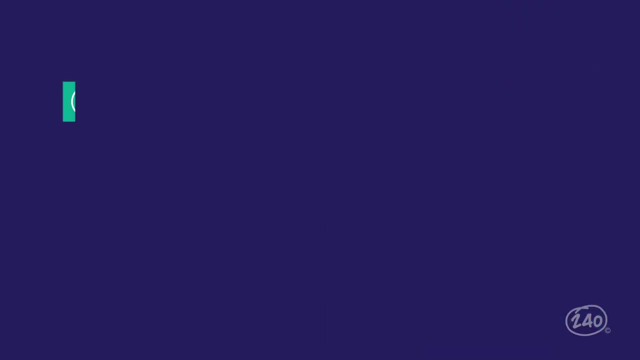 in the classroom to help young students understand them in a developmentally appropriate way. That would be something like participating in a class vote to teach the concepts of voting or democracy. Moving on to the next social sciences objective, economics and politics, This objective is all about making connections within social studies disciplines For this objective. 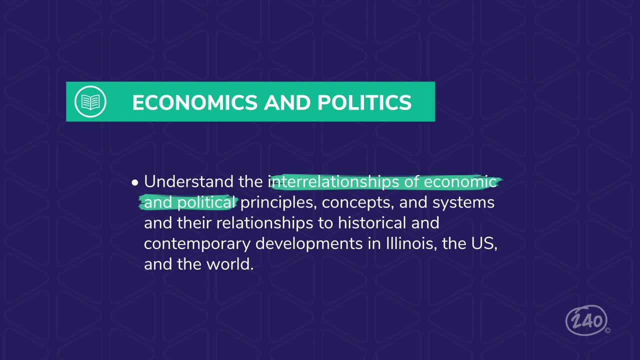 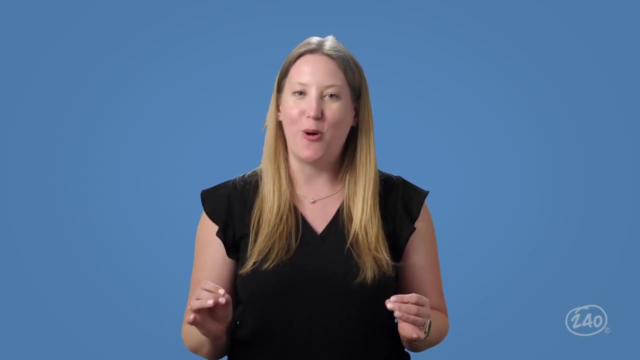 you will need to understand the interrelationships of economic and political principles, concepts and systems and their relationship to historical and contemporary developments in Illinois, the US and the world. Whew, that is a pretty broad scope for one little objective. 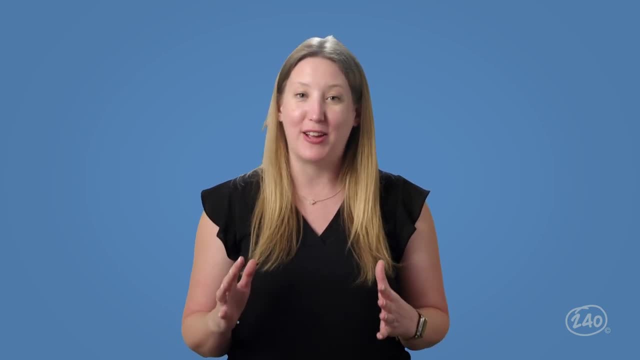 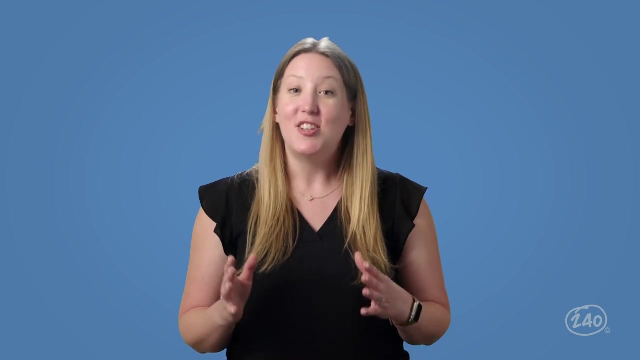 If you're like me and tend to feel overwhelmed when you see a lot of concepts squeezed together in one huge sentence, don't panic. Our study guides are designed specifically to help you break down these concepts into manageable pieces and draw connections across disciplines. Check out this video that's part of our study materials on the types of economic systems. 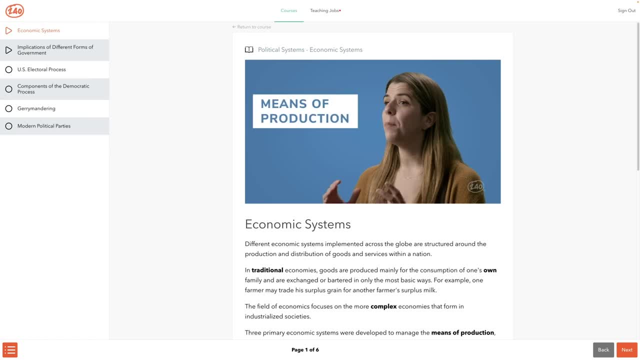 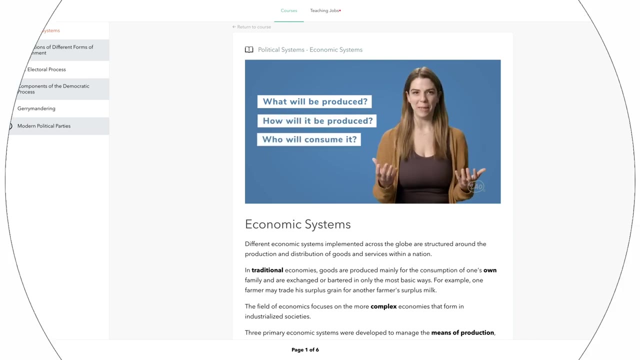 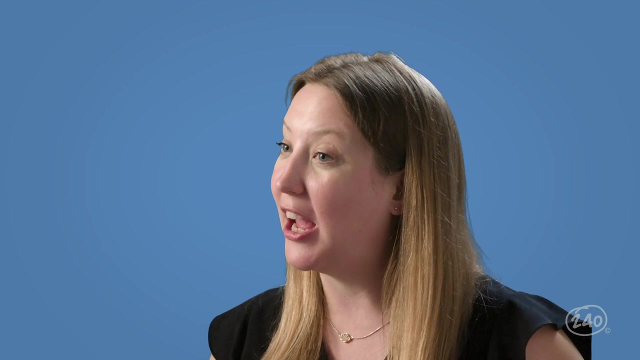 Three primary economic systems have developed to manage the means of production, which are the resources used to produce goods. The type of economic system implemented answers these questions: What will be produced, How will it be produced And who will consume it? Just like you saw in that video, questions for this exam will likely ask you to compare. 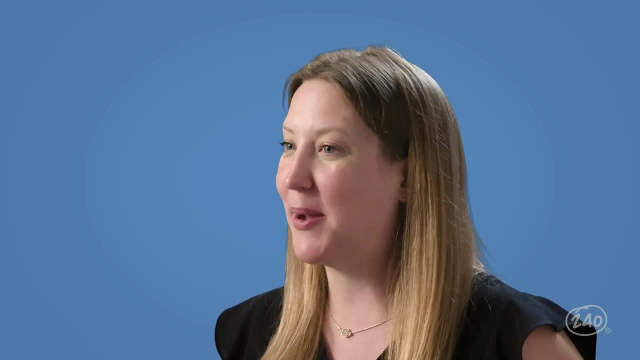 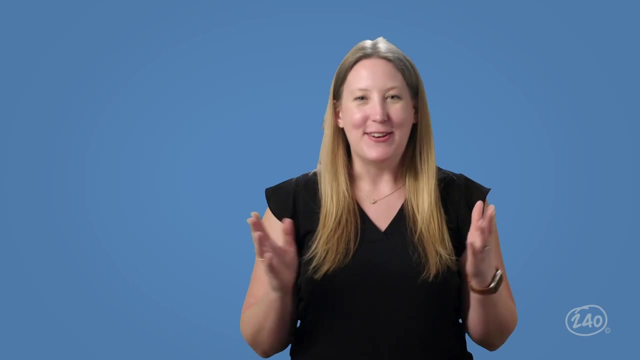 and contrast economic systems and explain the functions of certain economic concepts. But once it's broken down it's really not so scary, right? Okay, you're doing great. Let's move on to our last social science objective: geography and sociology. 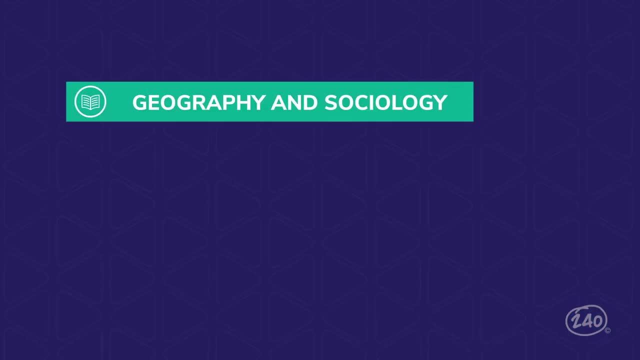 This one also focuses on connections within social studies. For this one, you'll be asked to understand major principles, concepts and phenomena of geography, sociology and culture, and the interrelationships between people and their environment. Now again, that may sound like a lot, but let's break it down a bit and see what we're actually. 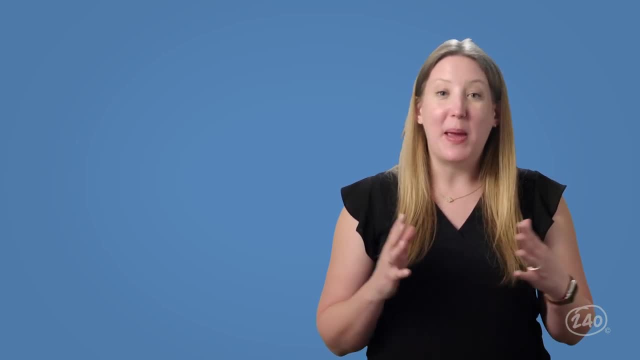 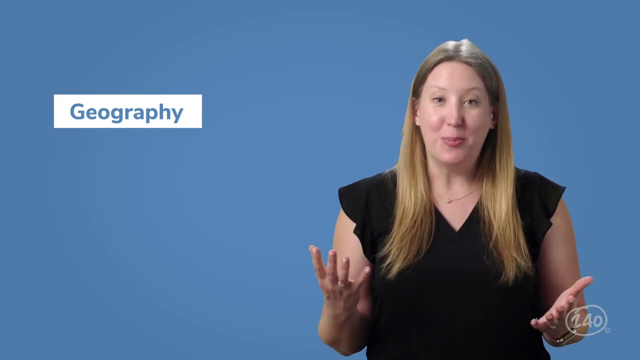 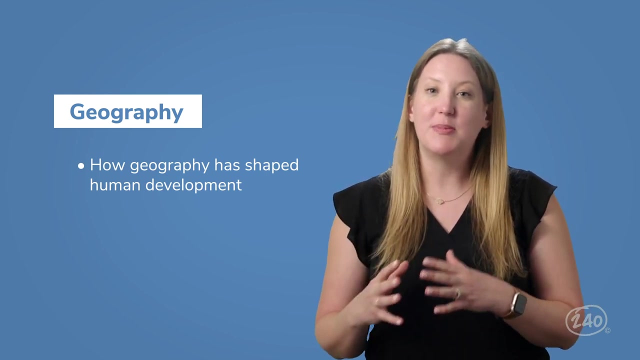 dealing with. A lot of this objective is just being aware of major physical features of Illinois, the US and the world and how to use a map or globe. Then we get into culture and sociology by talking about the relationships between human systems and the physical world we live in. These types of questions might focus on geographic 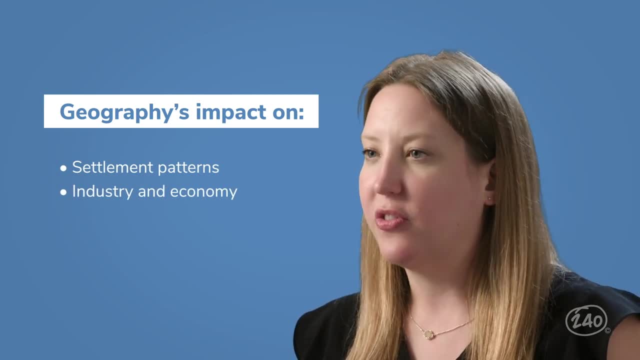 explanations for settlement patterns, how geography impacts major industries like farming, and how phenomena like droughts and floodwaters may be linked to geographic features of our society. First of all, you need to be aware of your own physical features. there are different ways to why you're far away from your natural world. 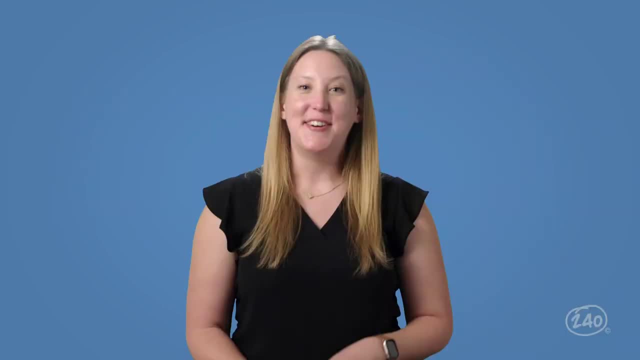 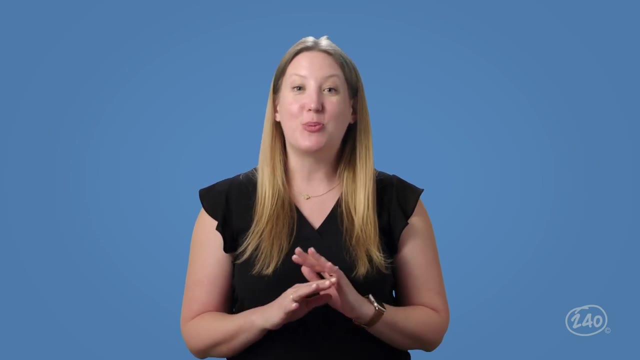 drought or famine have impacted human history. Okay, that's it for the social sciences. Let's keep it moving and head into the fine arts sub area, which is worth the smallest portion of your exam at 9%. Ooh sorry crew, that's not to say. 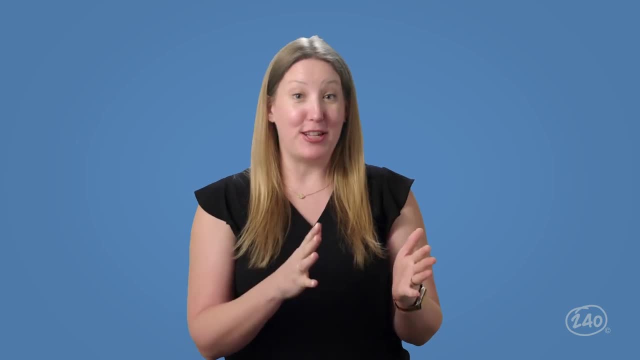 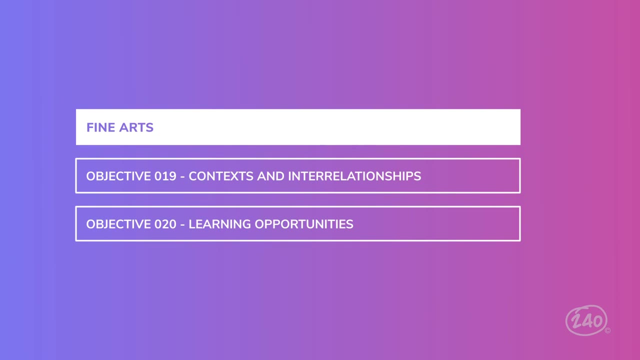 what you guys do isn't important. It's still worth about 13 questions on the exam. so let's get into what you need to know For this sub area. you'll need to understand the historical, cultural and societal context for the arts. 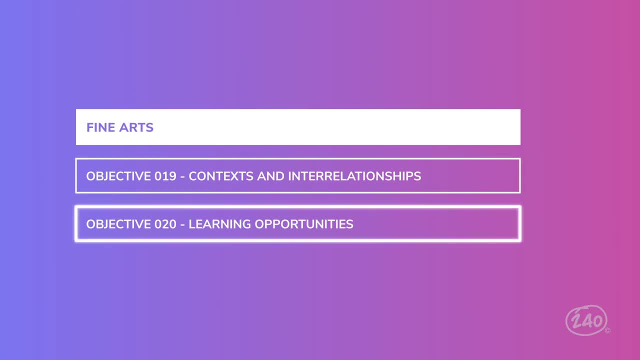 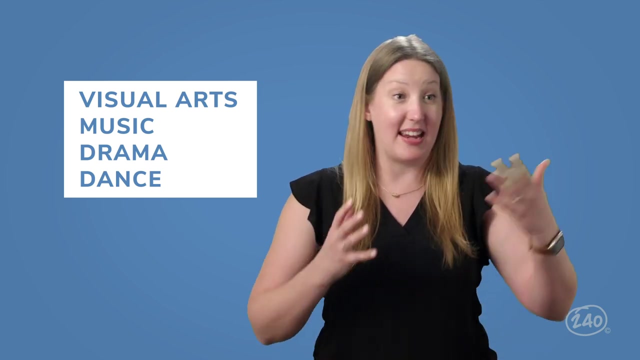 as well as the interrelationships among the arts and how to provide students with learning opportunities to engage with the arts through concepts, techniques and materials. And when I say the arts, I'm referring to visual arts, music, drama and dance and camera guys. 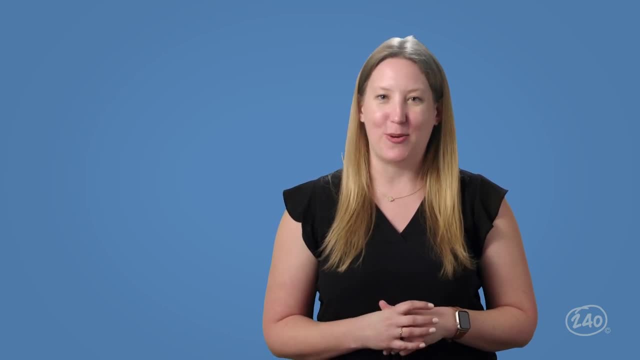 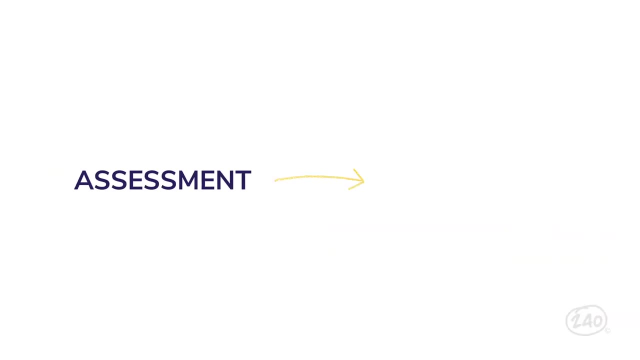 Lots of fun stuff. Part of what you'll need to know to answer the questions in this sub area correlates with what you'll need to know about teaching in general. For example, assessments should align with learning objectives- Not too bad, right. But you'll also need to know vocabulary and concepts. 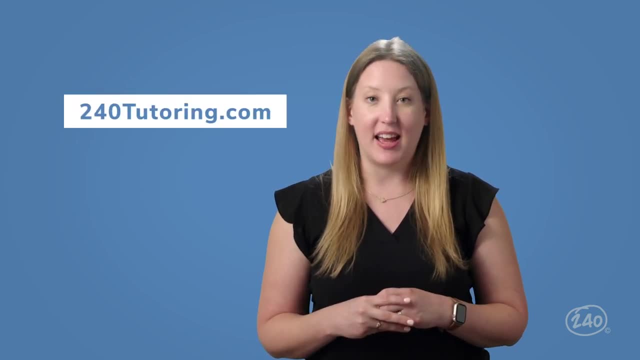 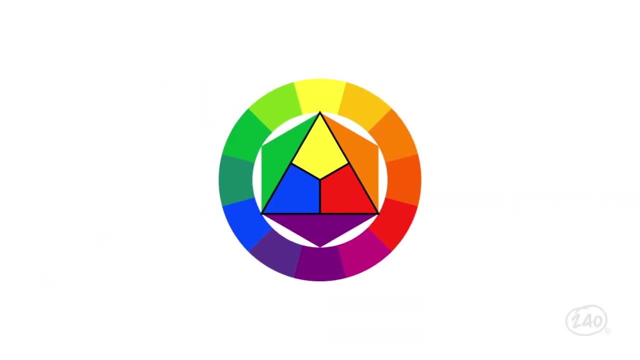 specific to the arts, which we do have covered in our study guide. but right now let's take a spin around the color wheel. The primary colors are red, yellow and blue. If you mix two of those colors together, you get a secondary color of orange, green or purple. 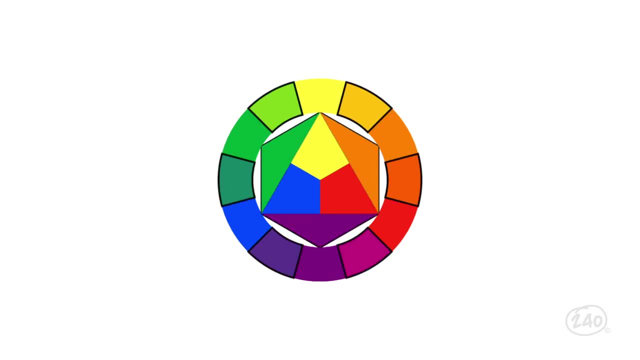 And if you mix a primary yellow and blue, you get a secondary color of orange, green or purple. And if you mix a primary yellow and blue, and if you mix a primary yellow and blue and a secondary color together, you get a tertiary color Colors across from each. 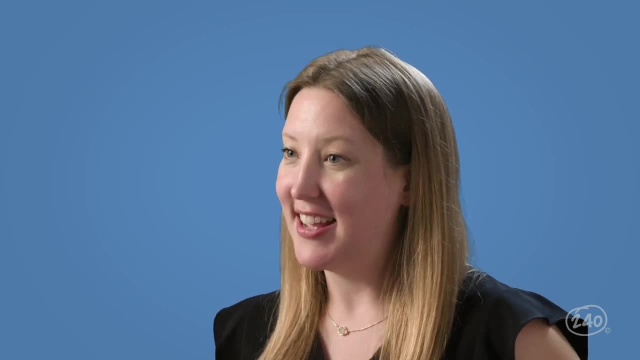 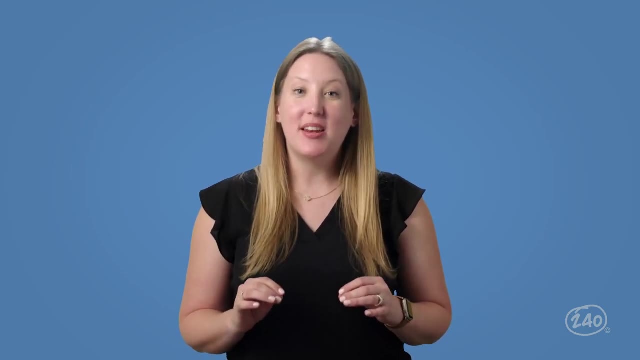 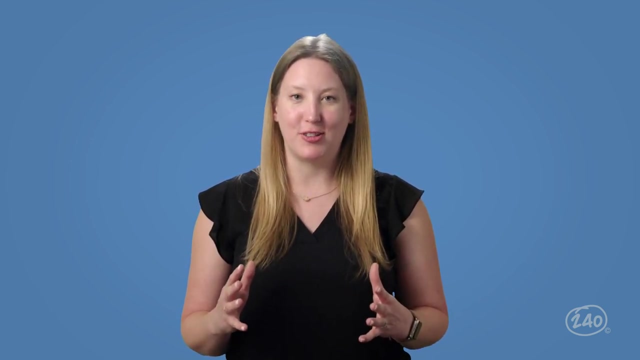 other on the color wheel are known as complementary colors. They enhance each other, really making their complement pop Alright. one sub area to go. This one is all about physical development and health, Just like science and social science. it's worth 13% of your overall score For physical development and. 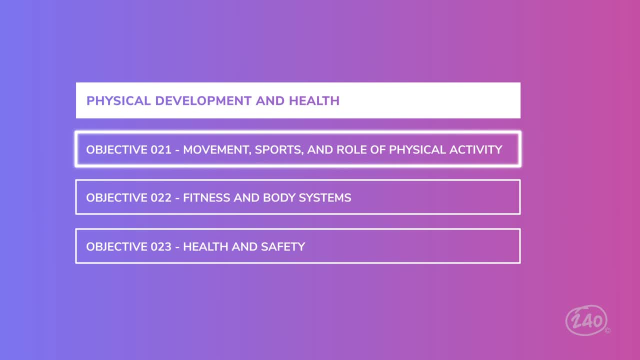 health. you'll need to know concepts and principles related to movement, sports, team-building, as well as the role of physical activity in promoting students' development. Systems of the human body, skill related fitness components and how they relate to each other, And principles related to health and safety and how to 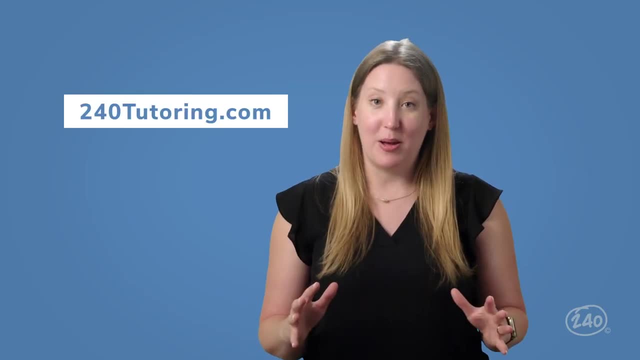 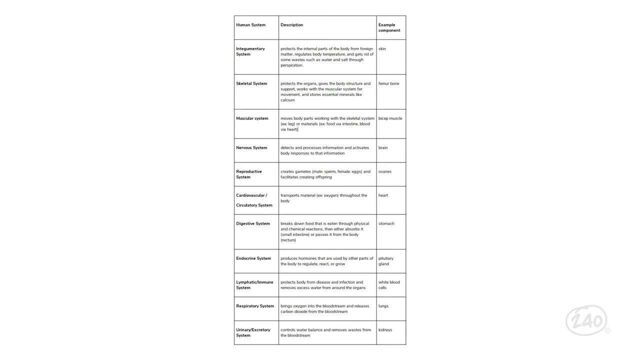 help students make healthy choices. There is a lot to unpack here, but check out what we have covered in the study guide. We have the essential human body systems organized in this handy chart, Along with corresponding flashcards and visuals, And that's just a small. 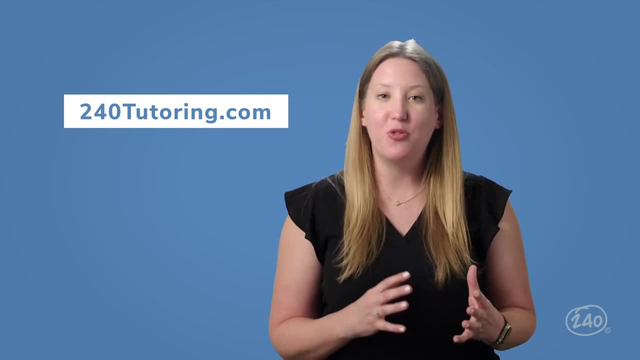 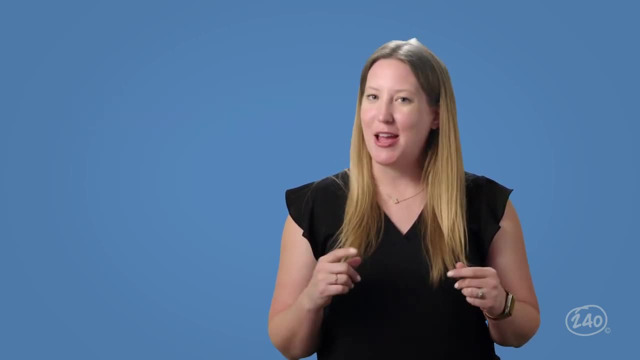 sampling. We have everything you need to know about movement, fitness and health covered in the guide. That was quite a journey we just took together. I bet you're ready for what's next, Now that we've gone over some of the big concepts. 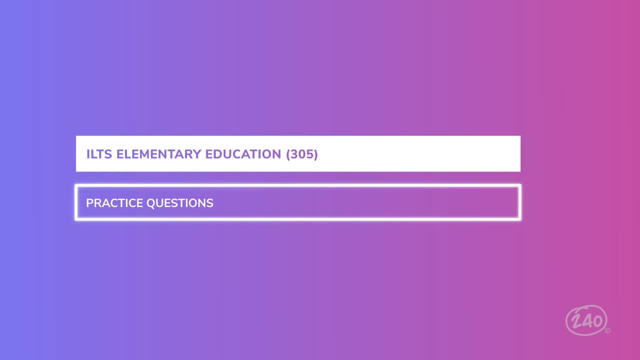 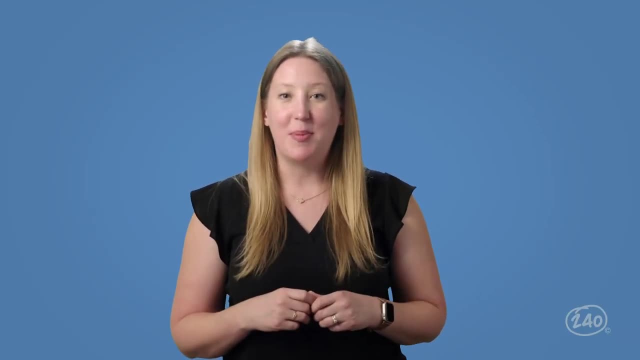 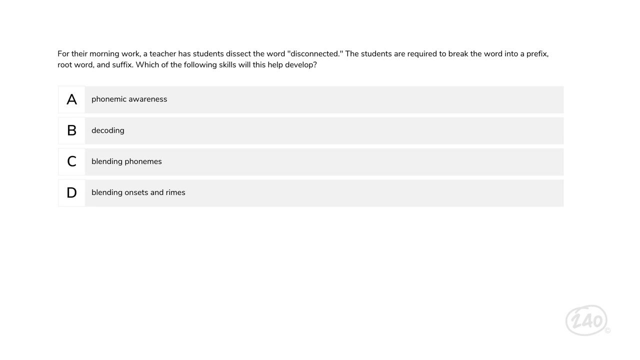 from each of our subject areas. let's look at some practice questions to show you how those concepts can appear on the test. Remember way back in the beginning when we talked about vocabulary instruction. Let's see how that's reflected in a question. For their morning work, a teacher has students. 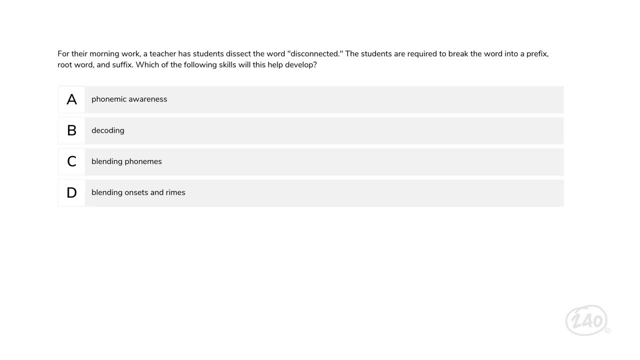 dissect the word disconnected, The students are required to break the word into a prefix, root word and suffix. Which of the following skills will this help develop? You may have identified this practice of breaking down the word as morphemic analysis, which is correct, And since using structural and morphemic 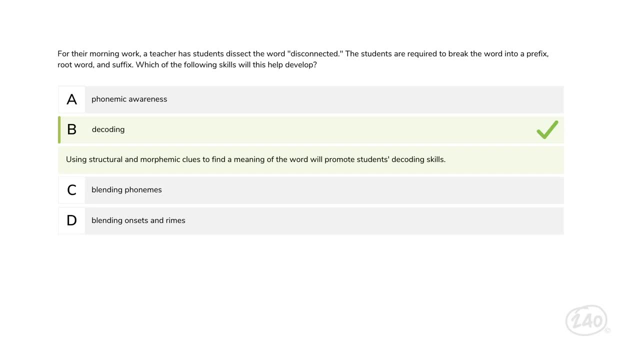 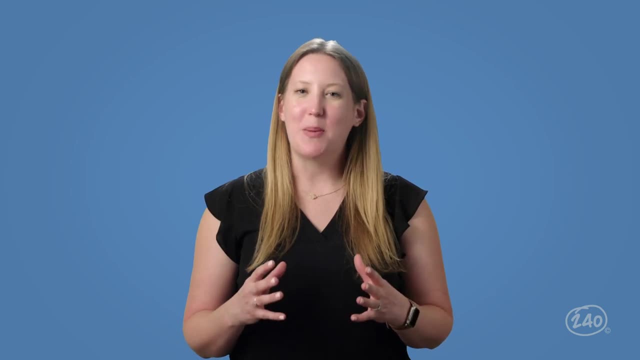 clues to find a meaning of the word will promote students' decoding skills. decoding is the right answer. Let's look at a math question. This one goes with the measures of center and range section. The number of inches of snowfall in Selbyville. 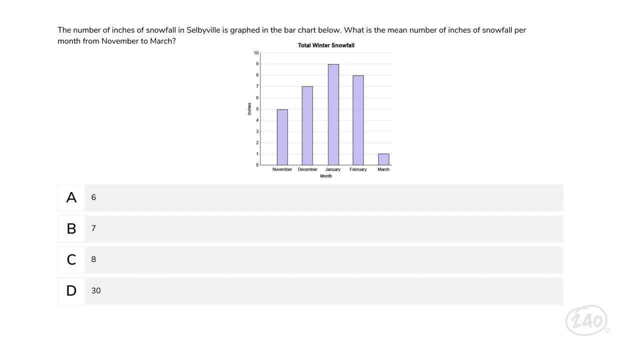 is graphed in the bar chart below. What is the mean number of inches of snowfall per month from November to March? To find the mean, we need to add up all the values and divide by the number of values in the data. So 5 plus 7 plus 9 plus 8 plus 1, which equals 30.. There are 5 data points, So 30. 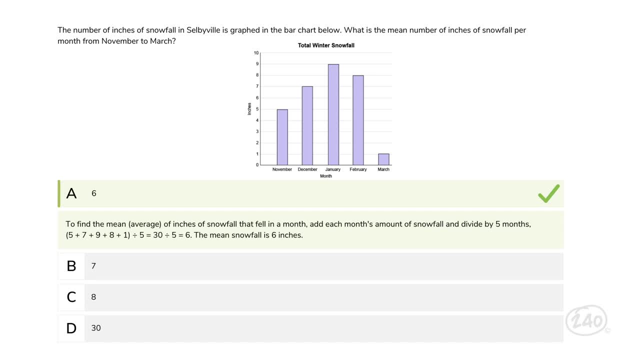 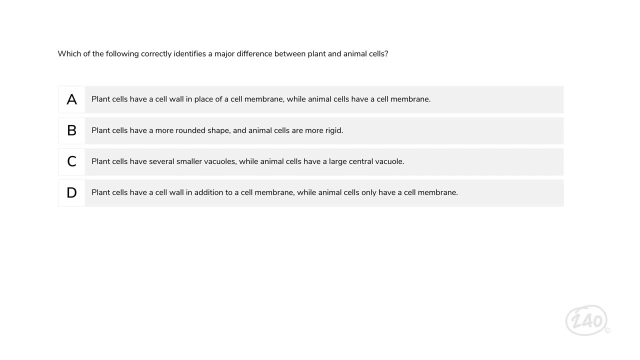 divided by 5 gives us 6.. So this one is correct. Next up, science. Which of the following correctly identifies a major difference between plant and animal cells? Let's look at these choices one at a time. A is out because it says plant cells have a cell wall. 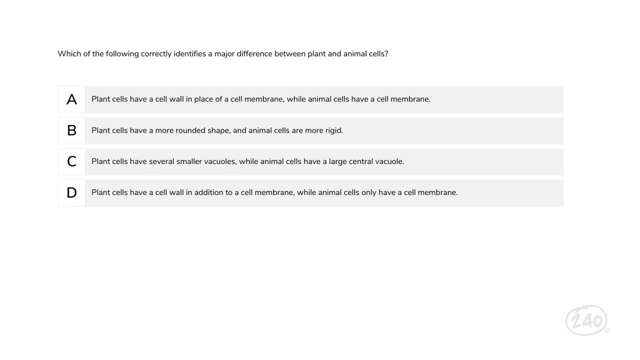 in place of a cell membrane, when really they have both. B is out, because animal cells are more rounded, while plant cells are more rigid. Again, in C they switch the descriptions. Plant cells have one large vacuole, while animal cells have many smaller ones, And that leaves D. Plant cells are more rigid due to their 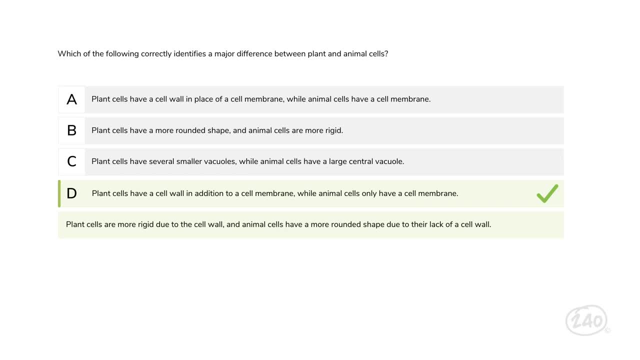 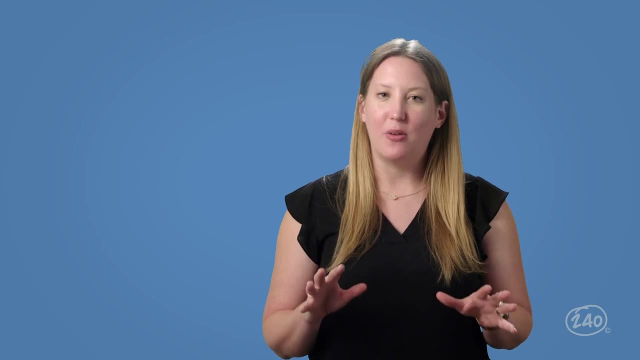 cell wall and animal cells have a more rounded shape due to their lack of a cell wall. Now let's look at a social studies question. Which of the following factors is most likely to encourage initial human settlement in an area? Okay, this may be a good time for a helpful tip For geography related questions. 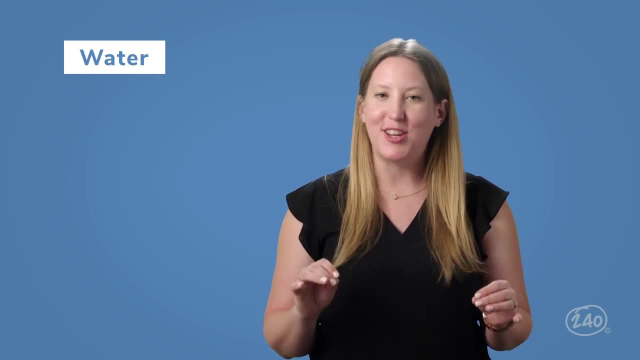 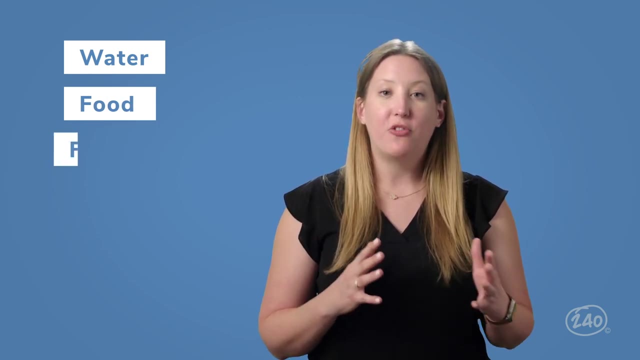 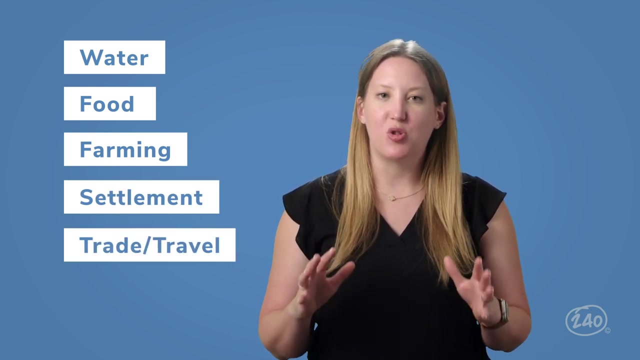 always remember that water is basically the key to human development. For the earliest humans, water meant plants and animals to eat. Later, water meant farming, which led to civilization and human settlement. Once we had farming down, water meant trade and travel, which significantly impacted human history. So let's read all these answers with water in the back of. 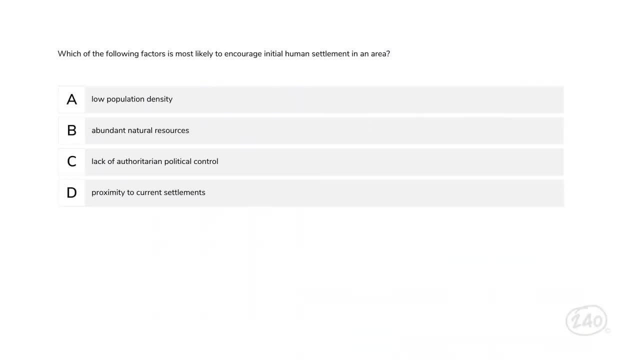 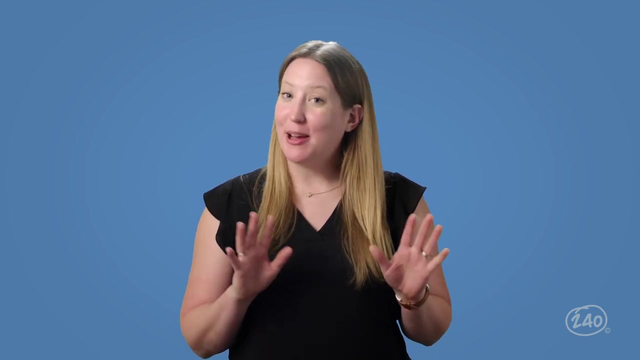 our minds Figuratively, not literally. Of these answers, only one is directly related to water, and that's B: Abundant natural resources. B is correct, Great work. Okay, now let's tackle a fine arts question. I know we talked about colors before, but